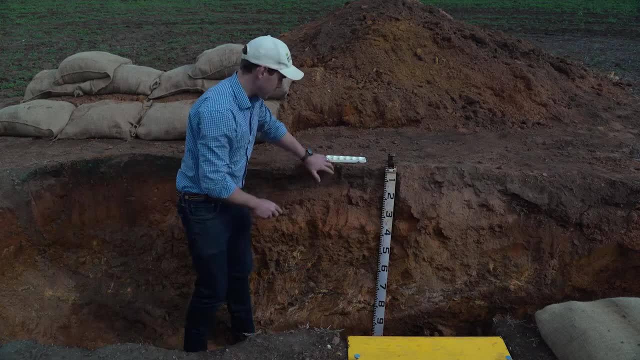 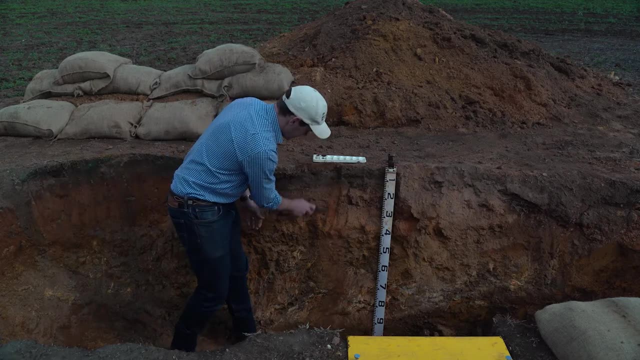 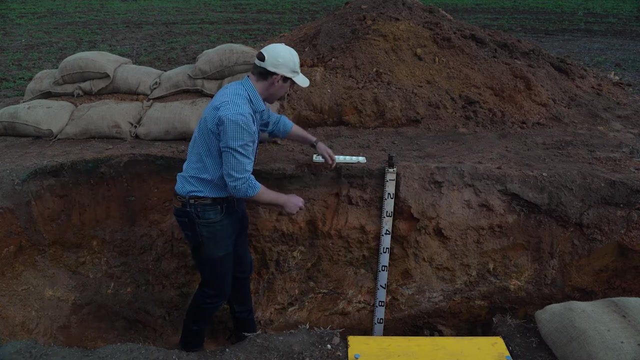 down through the profile and especially because we can start seeing what's called stratification, where we can get layers Layering out of that pH. Then we identified there's this change in colour which showed us this second layer. So again might do the up higher in this profile. part of the profile. put that in the tray. 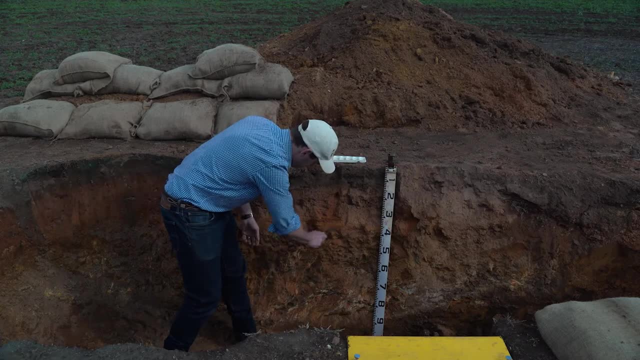 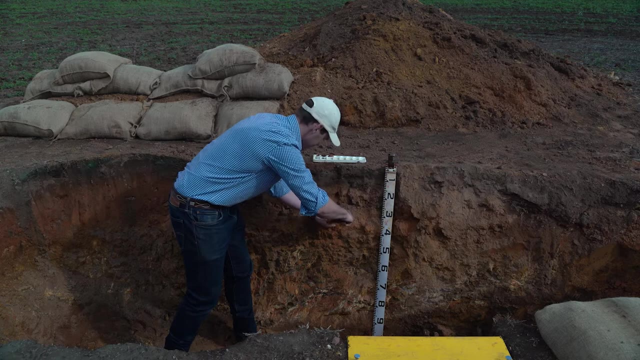 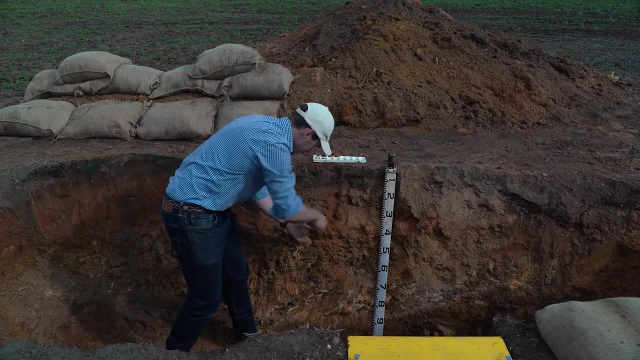 and then we might go down a bit further before work out where that change is down there. So sit above that, see if it's changed again, And then we can go down to this next layer which you can actually see. it's a bit harder. 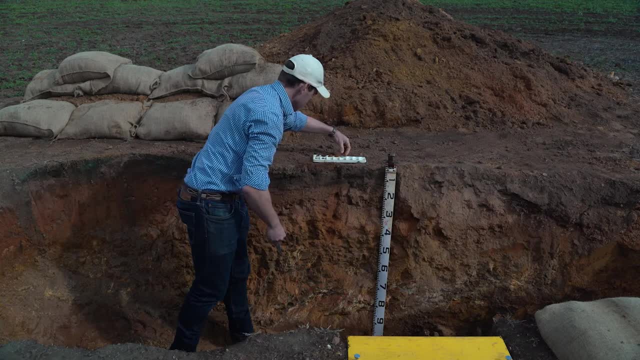 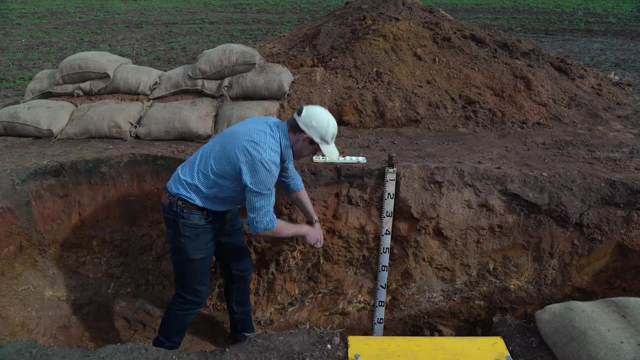 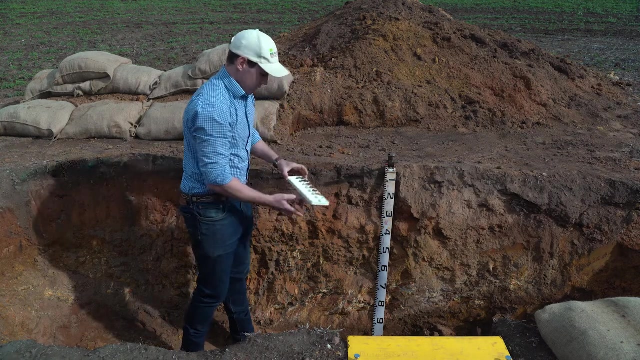 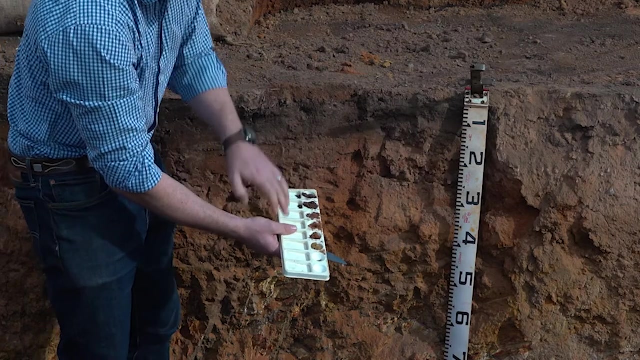 the clay content has increased. put that in there and then we can go down there, Down again into this subsoil, down further. So overall, there's your soil profile laid out from the top of the topsoil, bottom of the topsoil, top of that next layer, the bottom of that next layer, into what we've called. 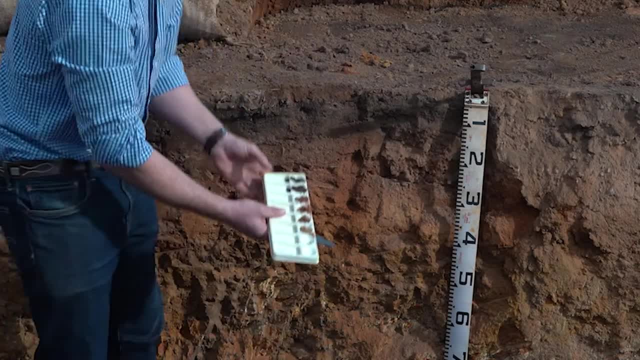 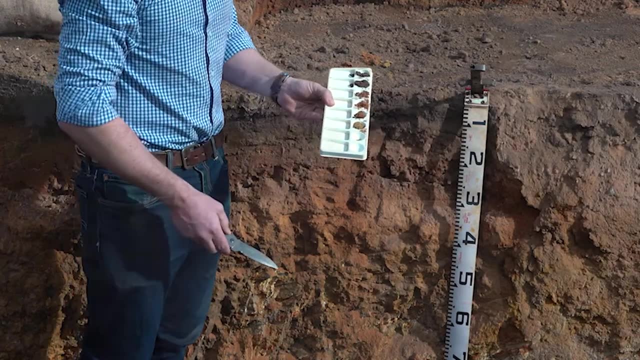 our clay layer and then into the deeper subsoil. So we'll now go and have a look at that for its pH and the changes and show you how to use the field techniques for identifying pH. So now we've got the samples that we've collected from the soil pit. 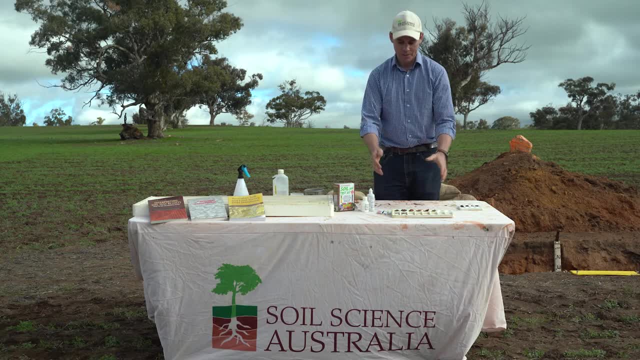 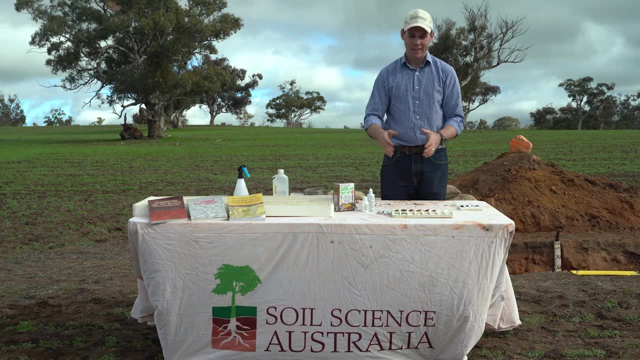 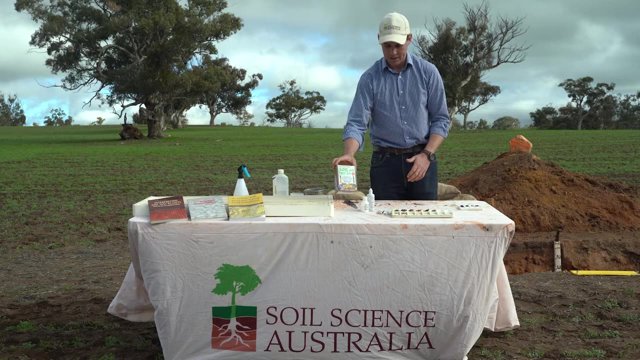 We now want to go through and do the field pH assessment, which the technique can be found in the Australian Soil and Land Survey field handbook which runs through the RALPAC and TUCKER method for that field pH. But kits are also commercially available and really simple for you to use in the field. 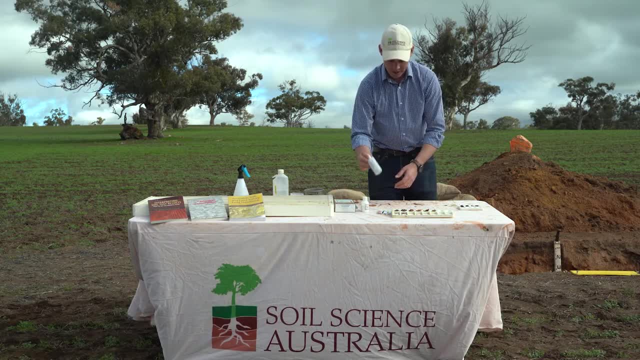 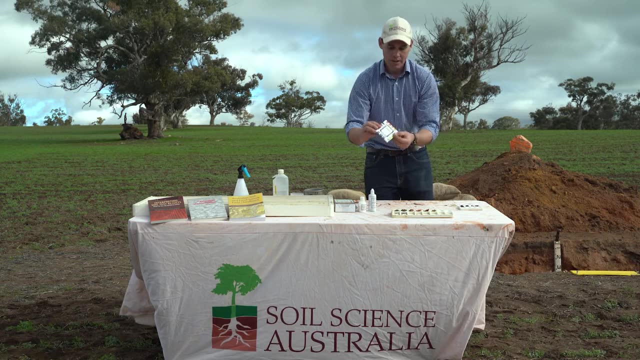 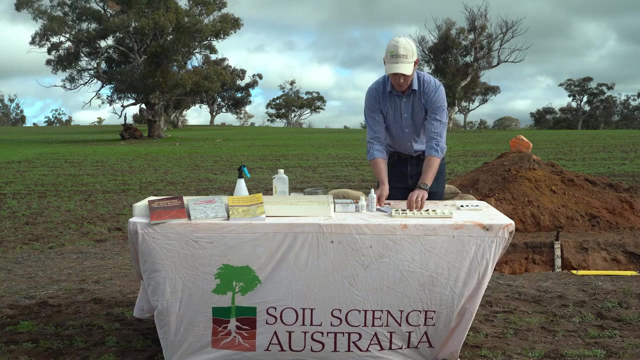 So in the kit there is some of the liquid dye, pH indicator dye, some indicator powder, barium sulphate indicator powder and a colour wheel. So this colour wheel will get you within about half a pH unit of your soil pH. So with that get the liquid solution. 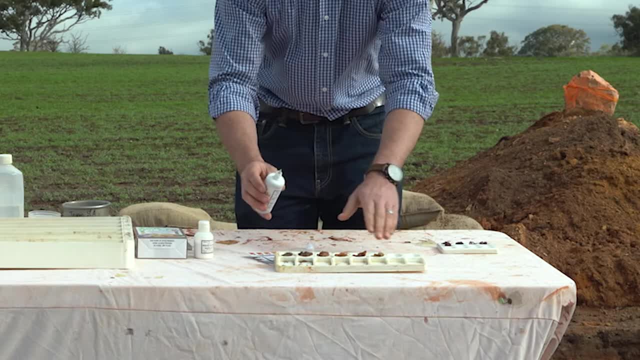 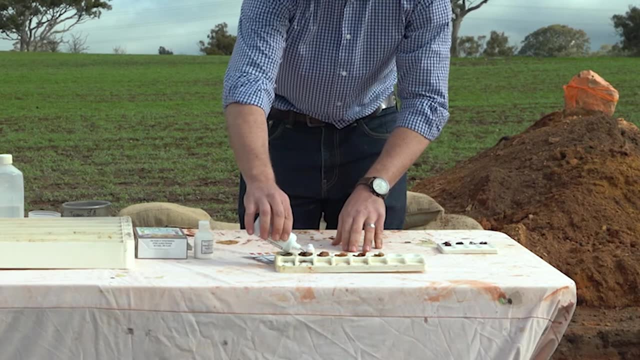 And, like we collected in the soil pit, we've got our topsoil working down through to our subsoil and we put a little bit of the solution on. This topsoil is slightly non-wetting, which is another challenge for us to work on in. 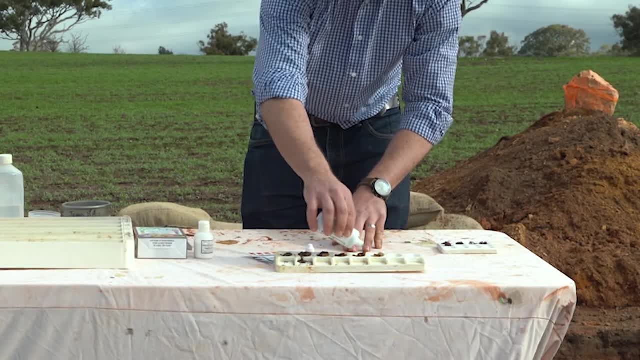 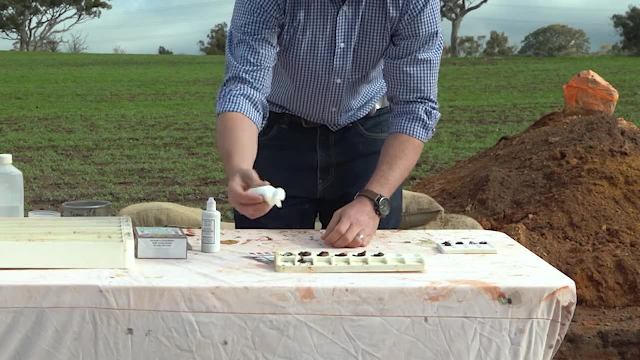 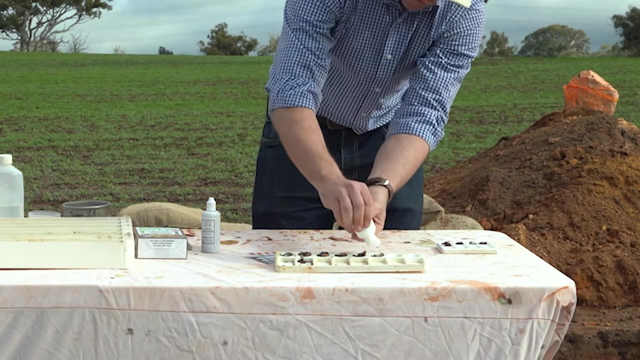 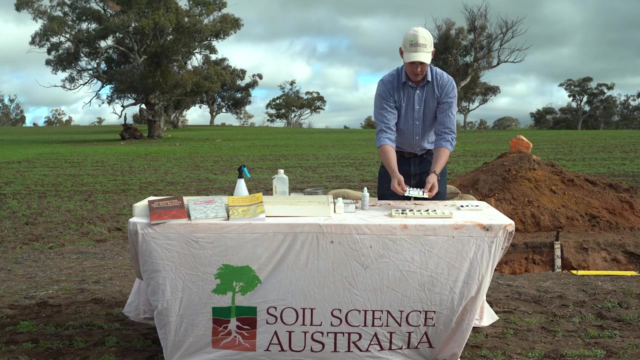 soil pits, We go down and put the solution on. We come back through and put the powder on top. So, overall, from the colour wheel, when we've got that laid out, we've put the indicator solution on and the powder, We then match up the colour wheel once we've left it to settle in. 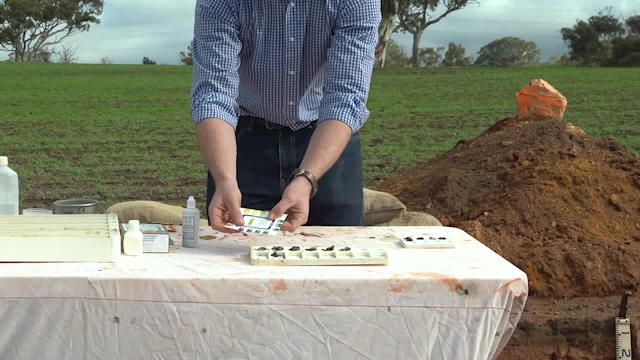 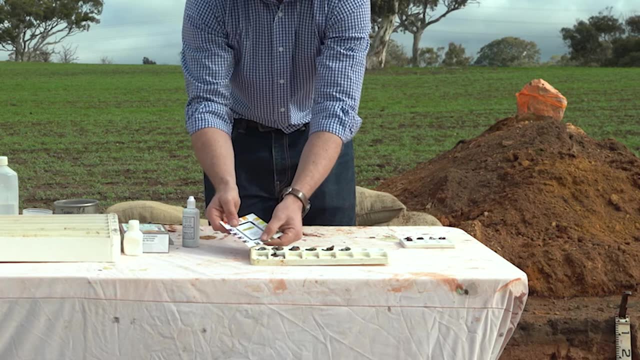 Then we can work down through the profile and line up this colour wheel with the soil. So in the soil here what we've got is actually close to 7.5-8 in the topsoil And then going down through a profile. So that was the top of the topsoil, And then at the bottom of the topsoil we're probably around 6. And then going down to the top of that next layer, we're around 7.. And then below that is about 6.5.. 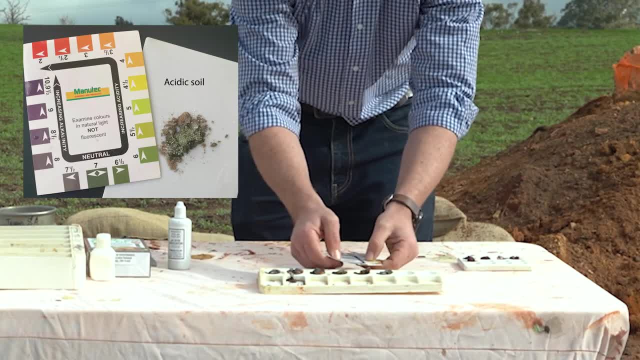 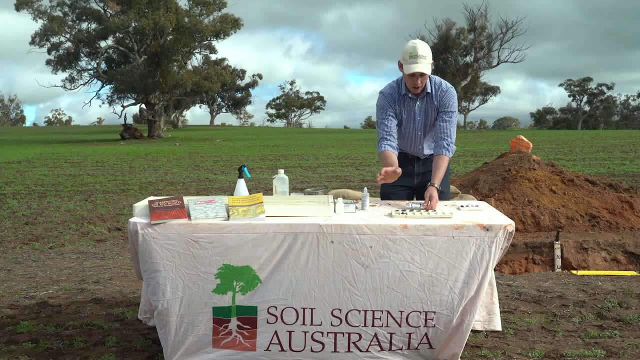 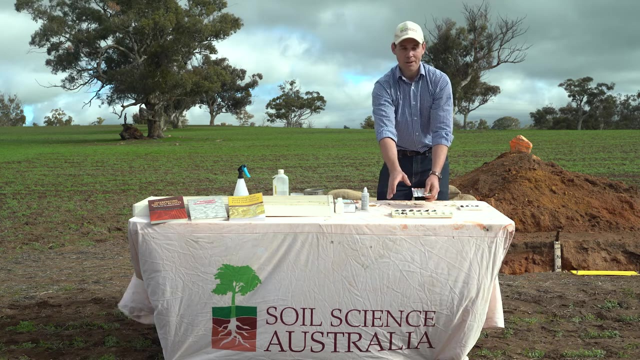 And then looking around that, yeah, 6.5. So around 6.5 down through the profile. What is interesting here? as we said, overall it's an acidic profile, So around that 6-7 pH. But the topsoil has actually been amended with lime this year. 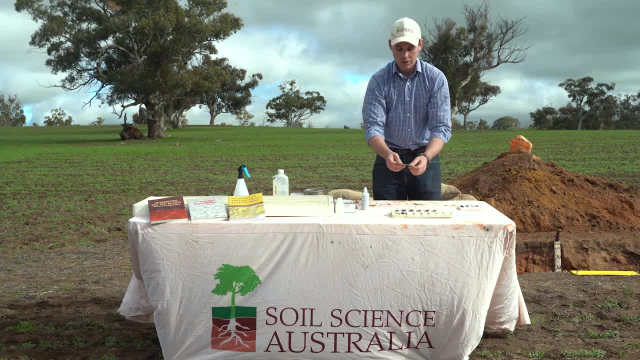 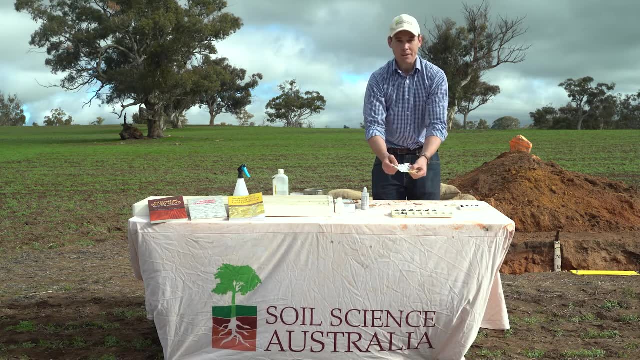 So lime is your common treatment for acidic soils. So when you use these indicators, especially if it starts getting down into the below 6, into the 5s, we need to be starting to look at a liming regime to amend that soil pH back. 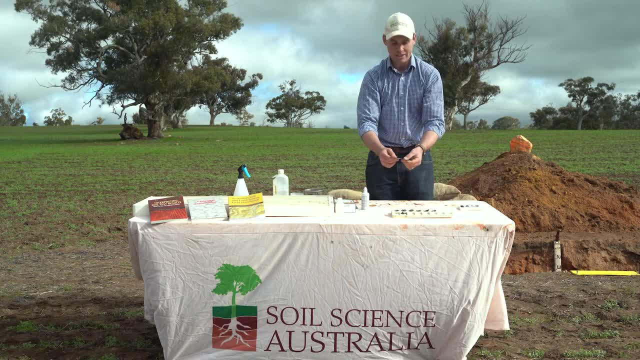 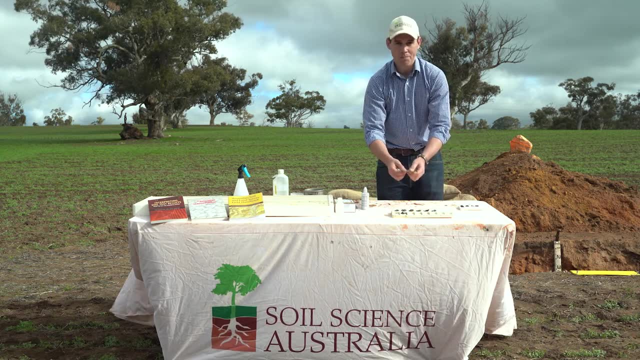 up to closer into that green, towards that 6.5 pH level. So the reason why we need to be applying the lime to increase that soil pH back to that optimum level is for improved biological activity. So that's the topsoil. So the topsoil is going to improve the soil activity and also improve nutrient availability. 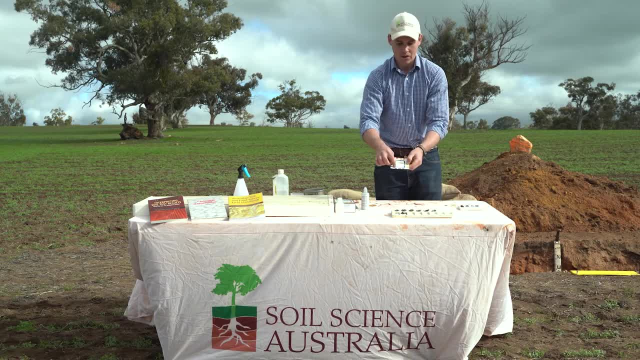 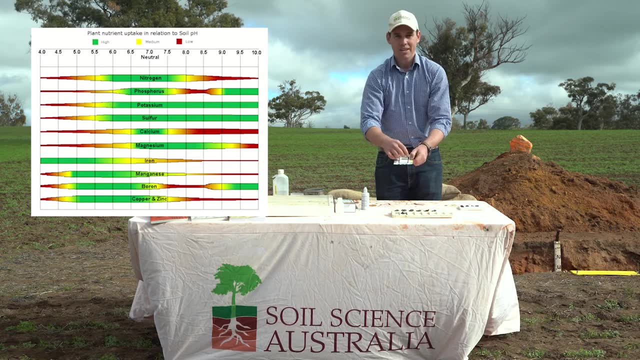 So nutrients will change their availability based on where they sit on this pH scale. And remember, when you are moving a pH number, it's not just one unit going from 5 to 6. It's a logarithmic scale, So it's going 10 times. 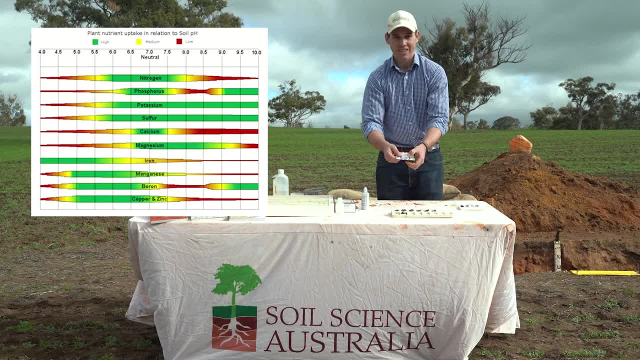 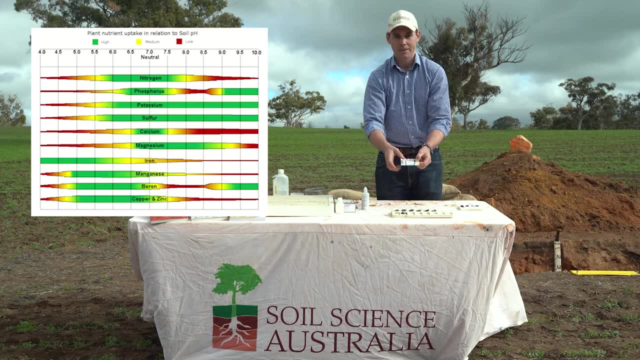 So 5 to 6 is 10 times 5 to 7 is 100 times more acidic or alkaline. So be aware of that that the small changes can have big impacts on how your soil is behaving and what sort of impact it's going to have. 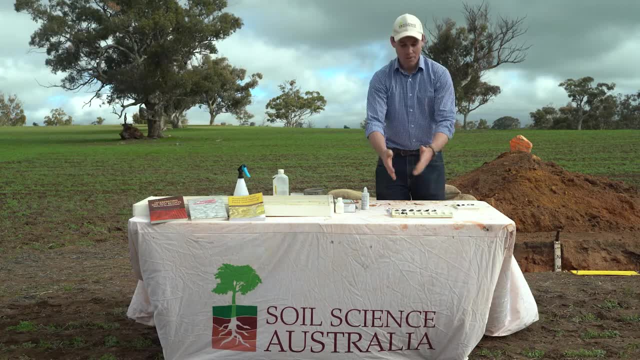 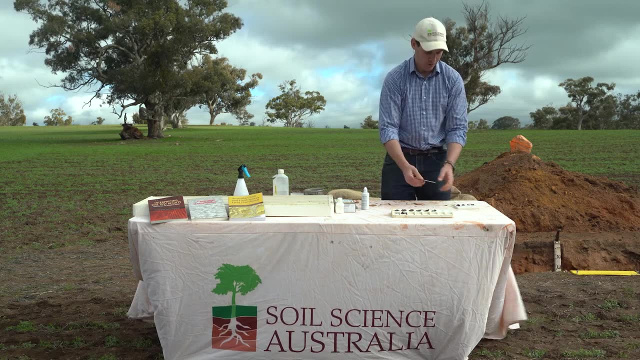 It's going to have on your plants growing in that soil. So, as you can see, we've had this acidic soil profile As a reference. we wanted to show you what it would look like if we had an alkaline soil throughout the profile. And here's one from a different area that is alkaline throughout the profile And you can see we've got soils pHs up around 8.5, even close to 9.. So really strongly alkaline. So, remembering the above 7 is an alkaline soil and below 7 is an acidic soil. 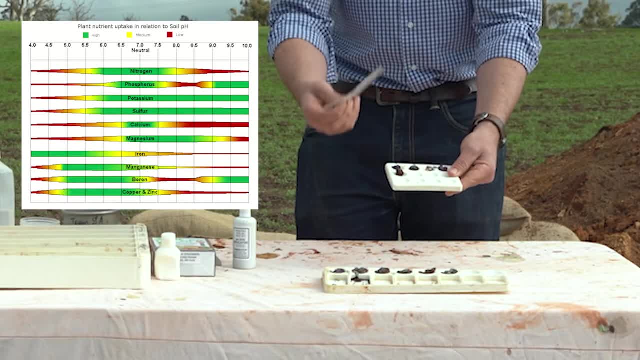 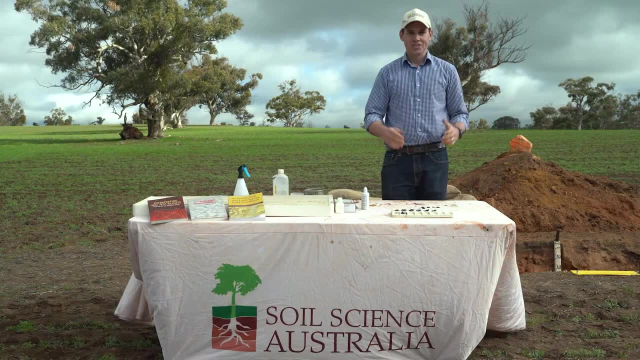 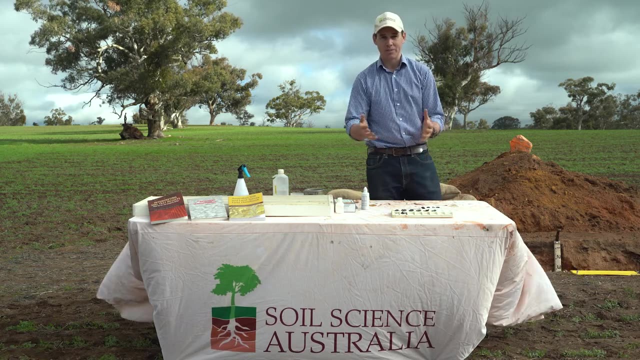 And the availability of nutrients, and how plants will grow and the tolerance of plants and the biological activity will all be impacted by this change. So here's an example how you can quickly test your pH down through your soil profile to understand why you might be having some constraints with your production in your soil. 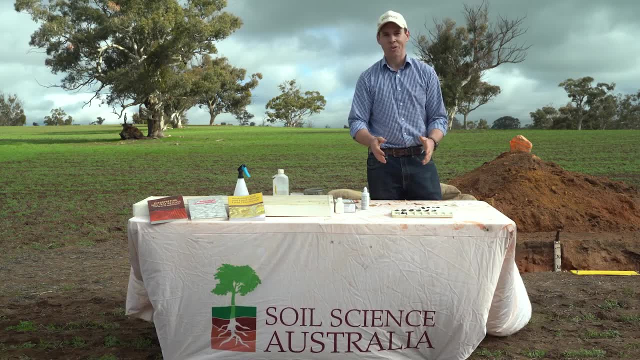 But for more information head to soilscienceaustraliaorgau. 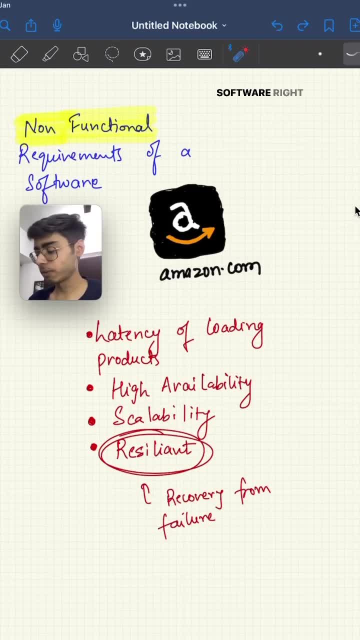 Let's try to understand this. non-functional requirements of a software, right? So whenever you design a system in software engineering, you need to list down your functional and non-functional requirements. Post that only you need to develop it or design it. So what are these non-functional? 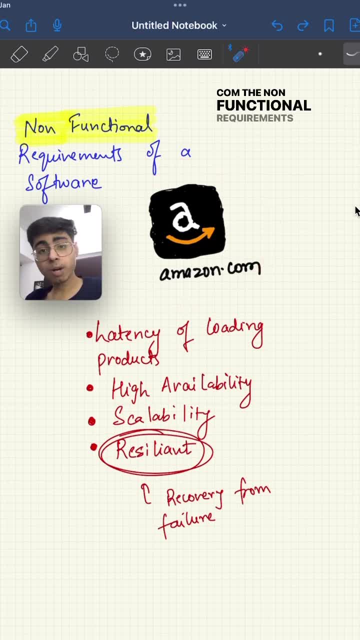 requirements: Let's say you are making amazoncom. The non-functional requirements will be that your system or your website should have lower latency for loading the products on the products page. right, People should not be waiting for too long to see the products. High availability: Let's say: 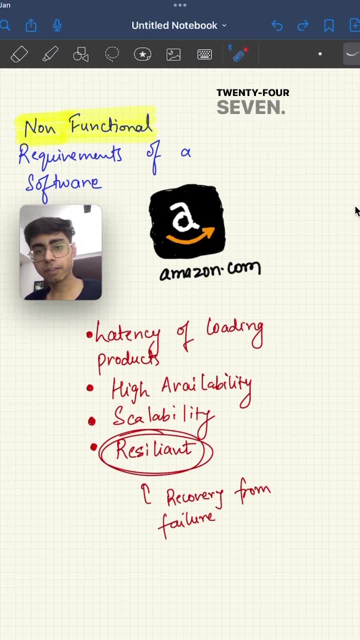 your website should be available 24-7.. It should not be like the case that on the night it is not there, on the day only it is there. So it should not be the case. Scalability: That means on some days, if there is some sale, then your website or your app should be scalable. It should be able to. 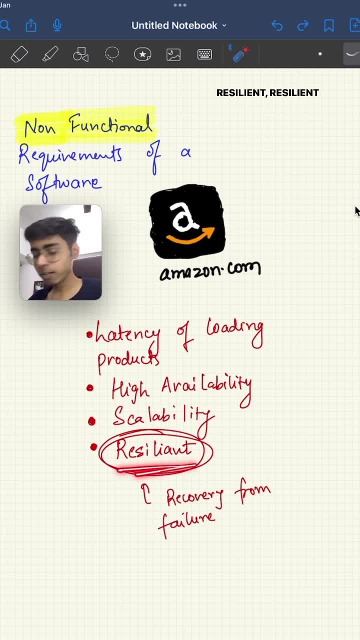 handle multiple millions of users right. Resilient. Resilient word means recovery from the failure, So if something fails, you should know how to recover it, or your system should automatically recover from that failure automatically. So these are the non-functional requirements of a software. 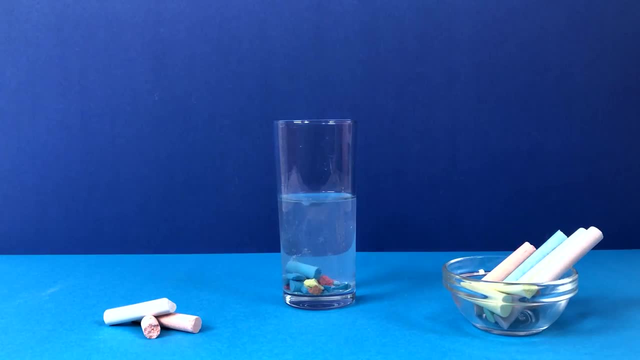 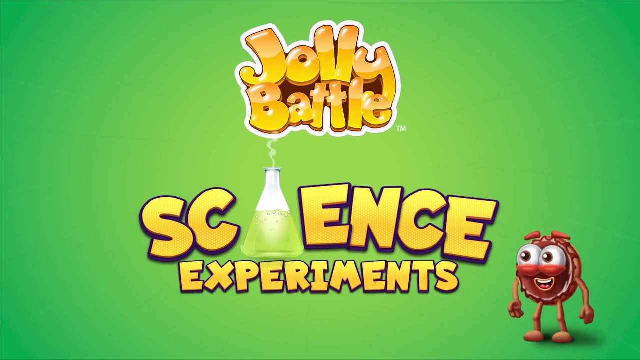 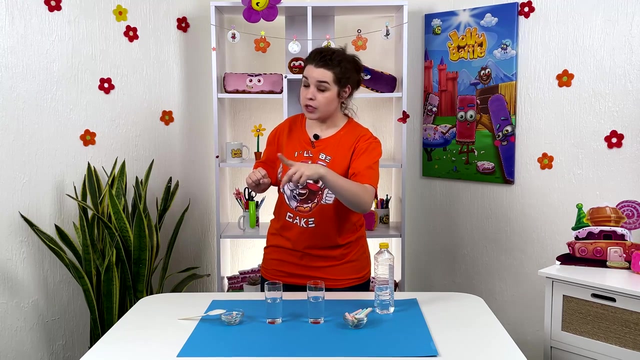 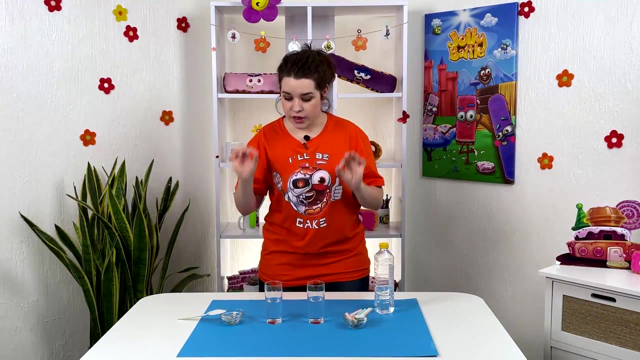 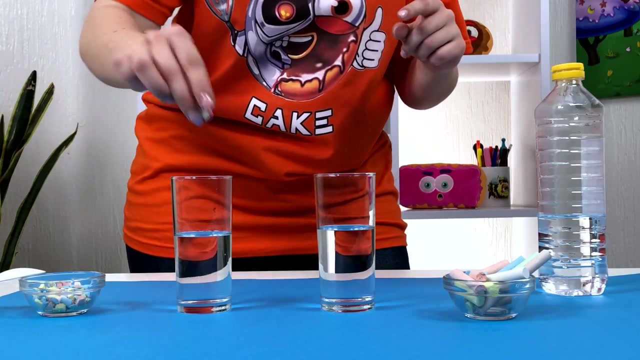 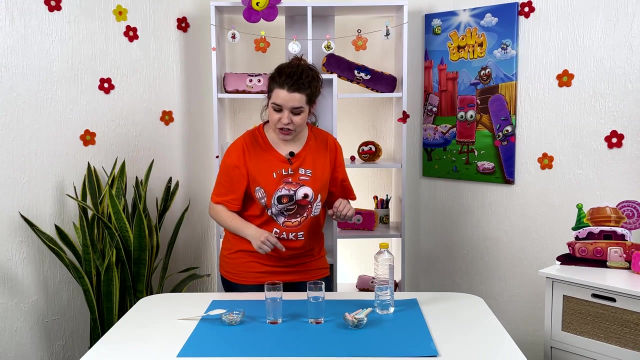 Hello friends, You are on Jolly Battle Science Experiments channel where we learn and experiment. Our experiments are often similar to magic. Look now at these pieces of chalk. I'm gonna throw it in there and they're gonna boil. But how and why I'm gonna tell you just right now.